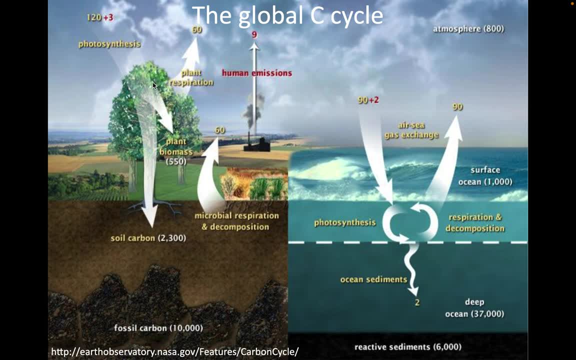 Human emission, But we also increase photosynthesis by growing farms and crops, Also by making the climate warmer. The growing season has increased in some places, But you can see this is still out of balance, right. But we're also adding more carbon to the oceans As. 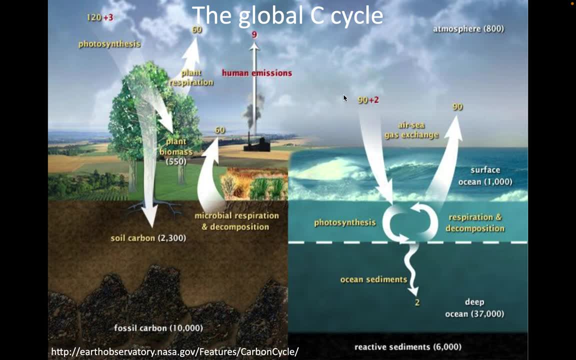 we add more CO2 to the atmosphere, a lot of that just naturally gets absorbed by the oceans, which then become more acidic over time. That's why they talk about ocean acidification. But still, if you add these numbers up right, we got plus two plus three. The system is: 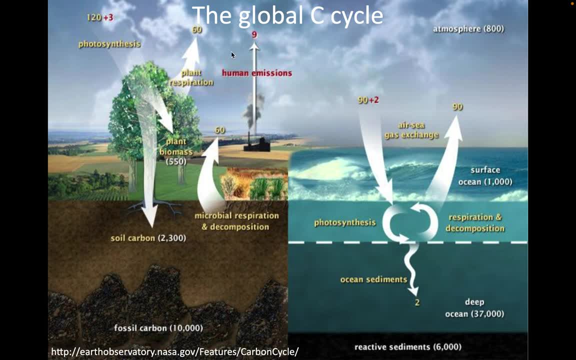 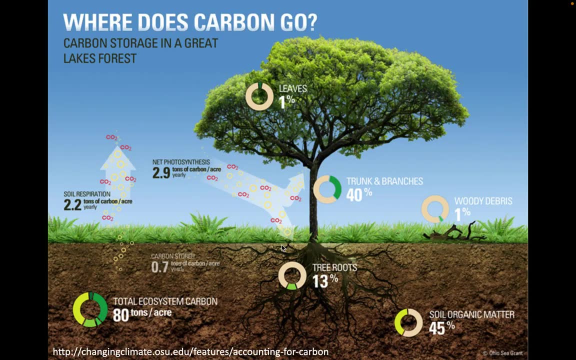 still not balanced. We're still putting more into the atmosphere than is cycling back out of the atmosphere, And that is why the climate is warming. Pretty simple stuff, Okay. so now we have a zoomed in system of the Great Lakes region, I believe I thought 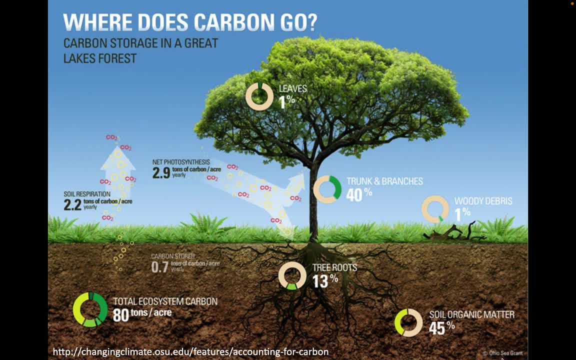 I saw this was like in Ohio or something. Oh yeah, Ohio Sea Grant. They're not by the sea. What are they funny? Anyway, our first task, I believe, is to look at where the most carbon is stored. We can see 1% in the leaves, 40% in the trunks and branches Makes sense. 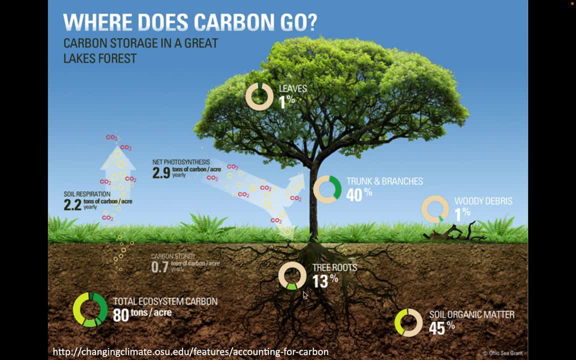 There'd be a lot more there, 1% in woody debris, And then hopefully you find, wow, actually most of the carbon is in the soil in a forest, And so that's, just like Mike says, right, We don't grow crops, We grow soil, and the soil grows crops. Just like in this forest the soil is really. 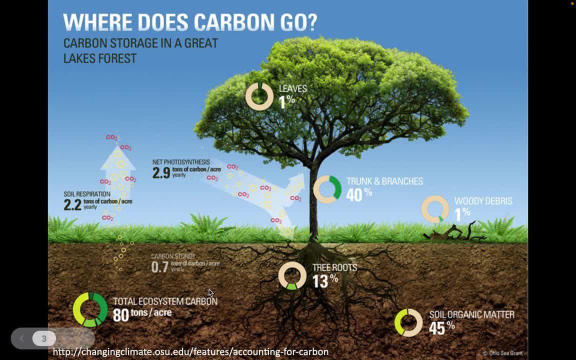 providing everything else for the whole forest. Our next one is to look at the soil respiration compared to the net photosynthesis. right, How much carbon is coming into this system? How much carbon is leaving this system? And so we see 2.9 tons of carbon per acre per year. 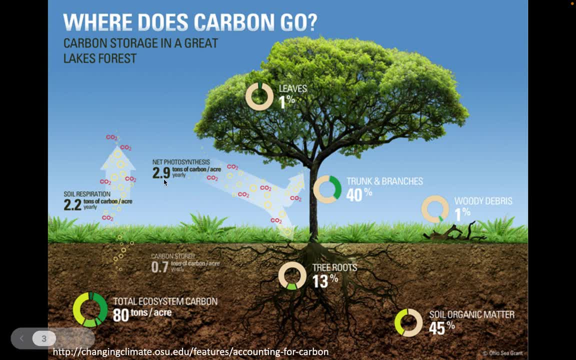 entering the system through photosynthesis And that's after respiration, right? That photosynthesis, Some of that carbon doesn't enter The system because it's just lost during plant respiration And then 2.2 lost to soil respiration. 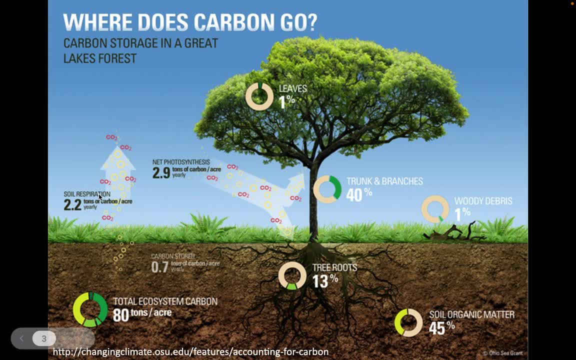 So the question is: you know which one's greater, where you have more coming in than going out? So what happens to all of that carbon that's going in? Well, it's actually stored in the soil. Here it is: 0.7 is the difference between those two. So this is, at least in the forest, the breakdown of carbon. 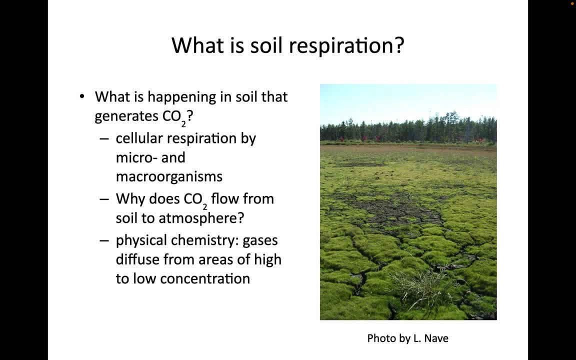 So the soil respiration is on the soil. So if you look at this situation- we're going to look at basically data of soil respiration in this forest throughout a whole year- So what is actually happening that produces CO2, so, just like we saw in this last one, we have a respiration. 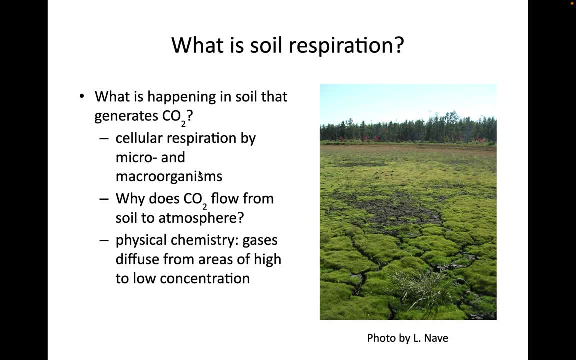 So all these microbes, and actually microorganisms in the soil, are doing cellular respiration, releasing CO2, even if they don't have lungs, Whoops, you still do cellular respiration. That's why breathing is not really the best option, best term, you know. but uh, that's how we release all that extra co2 from our own system. um, and. 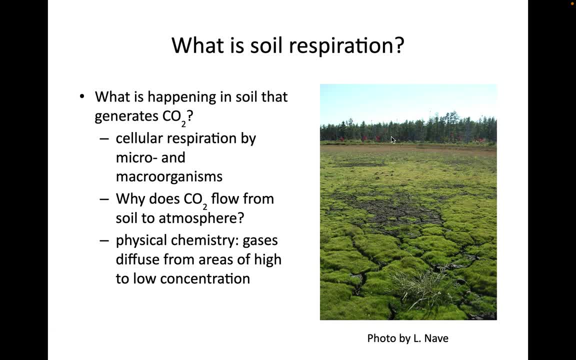 then the question of once it's in the soil, why is that getting released to the atmosphere? um, what we saw in the last situation: right, there's a little bit extra carbon stored here. um, so if you remember from chemistry last year, if you have, or two years ago, if you have higher density of, 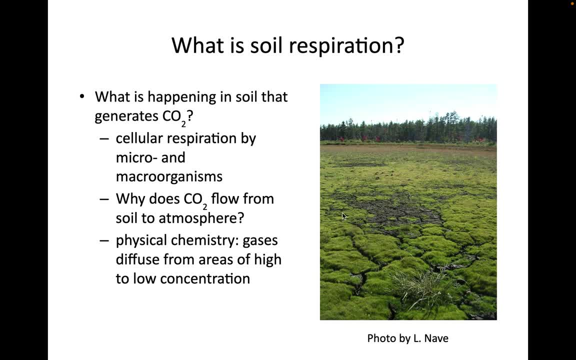 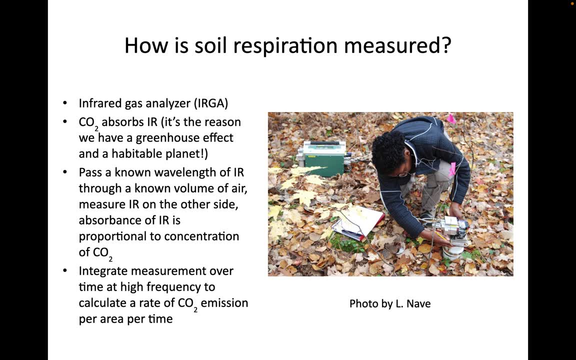 gases. they will diffuse to a lower concentration, um, just because you know gases like to fill the space. um. so, uh, how is this data measured? um? so here's the equipment they used: infrared gas analyzers. basically, co2 is an absorber of infrared radiation. infrared is what you see when you put on. 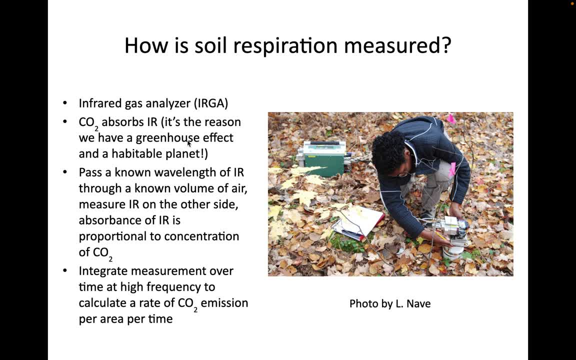 heat goggles and that's actually the reason that we have the greenhouse effect. carbon dioxide absorbs infrared and then actually jiggles a little bit and re-releases it um. so basically you can shine infrared through um and if you have a different amount of infrared on the other side, you know. 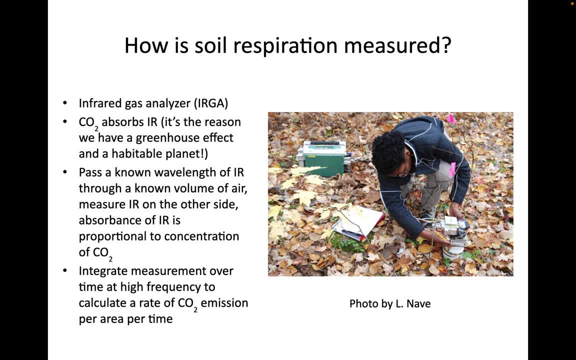 that some of it must have been absorbed by that uh carbon dioxide in there, and then you can therefore measure how much carbon dioxide is in the soil, um, and so we're going to zoom in on the little thing underneath here. so, yeah, it's basically like a little uh, you know we're trying to trap. 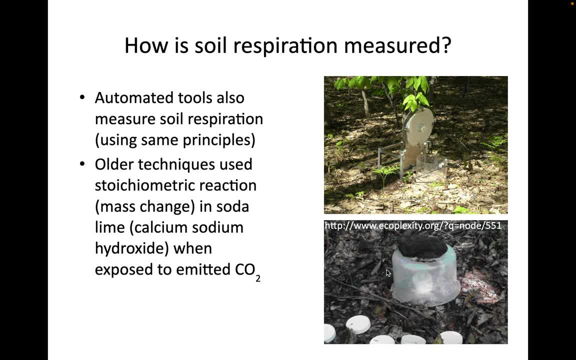 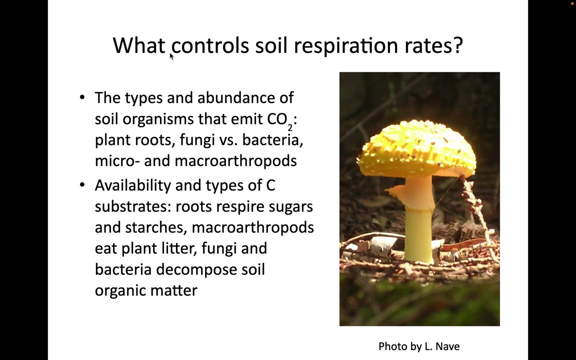 the air coming out of there. um, so then we can measure carbon and carbon dioxide. um yeah, so the new ones are just totally automated. so that's why you can have it be released, sort of sort of versus trapping it, the old yogurt container. um, so how is this, uh, controlled? how does it increase or decrease? 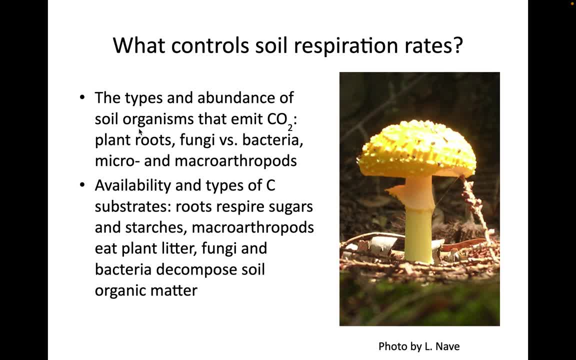 um, so, depending on which order you're using, it's going to be a little bit more difficult to measure. um, so i'm just going to covered that up with this hat. um, just informal. um, if you're adding more nutrients in that case, or if you have more. 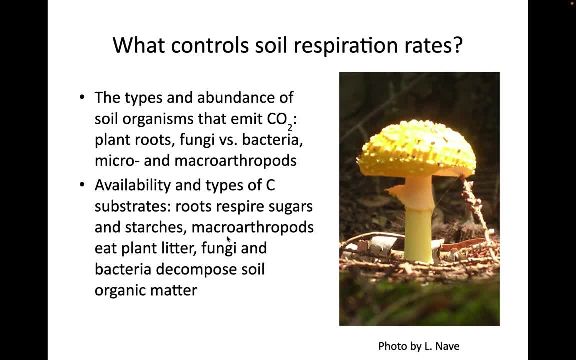 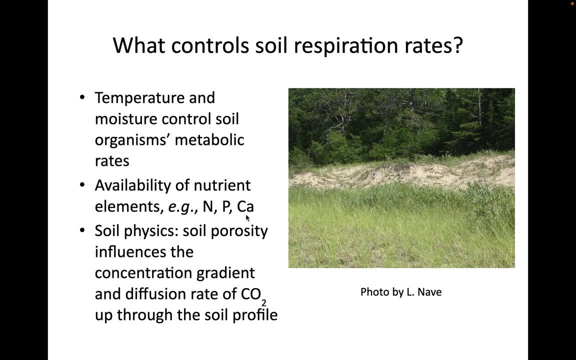 ummy, like some kind of oxygen Jared actually, like you know what it's your the plastic table i was organisms decompose or digesting that material. let's see. and then temperature and moisture: these are actually two variables that you're going to graph and you are going to see how that affects soil respiration, but basically same way. 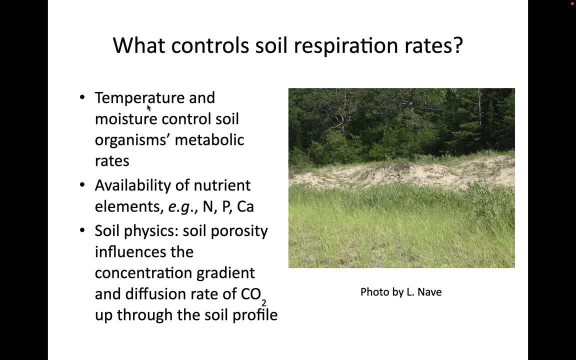 they affect you. all the microbes do the same thing. I've heard. I don't know, I don't know how true it is. I've heard a few things. you know the smell of when it rains. I've heard that it's either the ozone that comes down from the upper 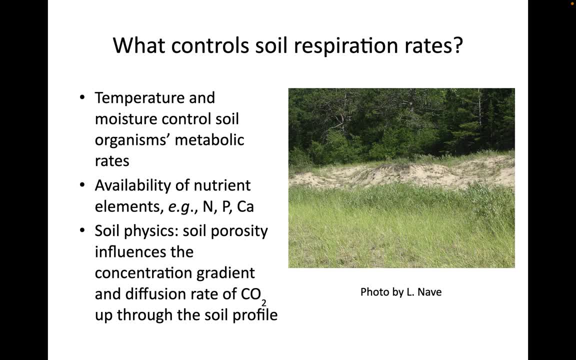 atmosphere, or I've also heard that the smell of rain is, is the microbes in the soil are more likely to be alive. so one of those two things. maybe it's the moisture controlling their metabolic rates. there's more nutrients, huge limiting factor, as always, and then the characteristics of the soil rate. 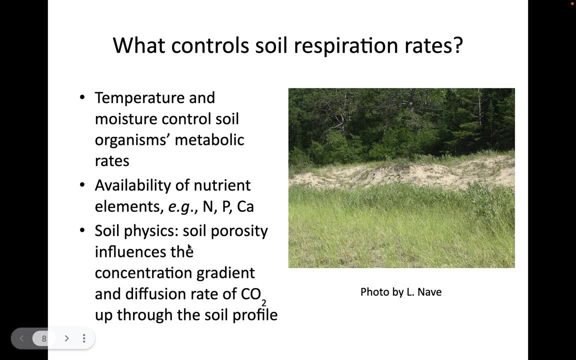 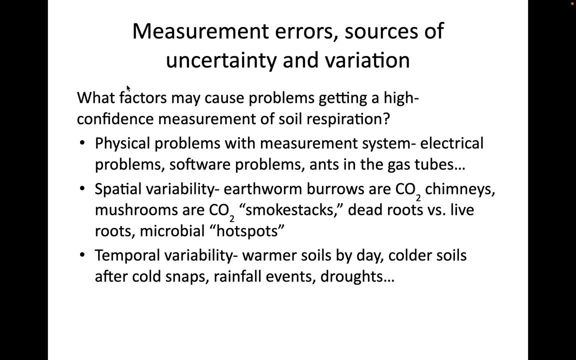 porosity is the spaces in the soil. if there's not any spaces for the stuff to live, not going to be a lot of respiration, let's see. so these are some of the issues that they might have with with their data, which is still post-modern global climate, which is, yes, it's actually good to be able to. 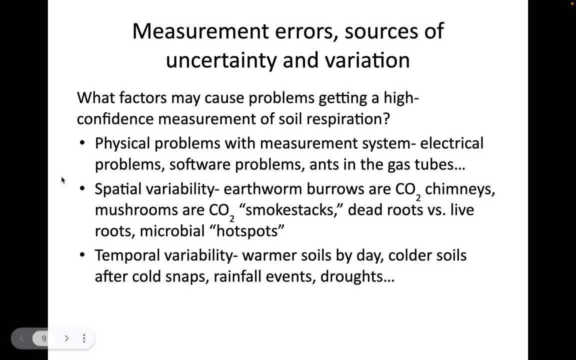 use drained water right now. there's a few things that you want to get into. when you're putting the soil down, that gear in because it'll as long as you get off land and the soil isn't going to get all the way down to the bottom of. 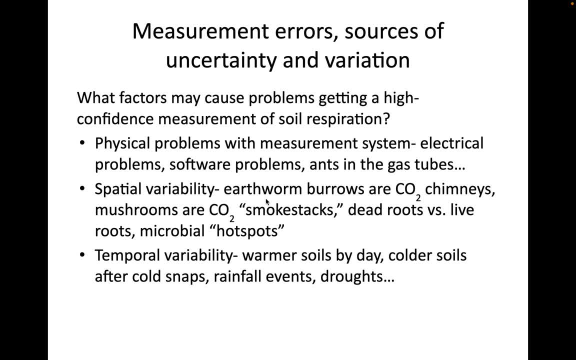 the earth's surface, it can still have issues with that soil right, so be careful of water. you can see a lot of the polluted soil that's going down there, and so that means it's a lot of animal material that's going to grow and it's very hard to get the soil out of that soil. that's going to be a lot. 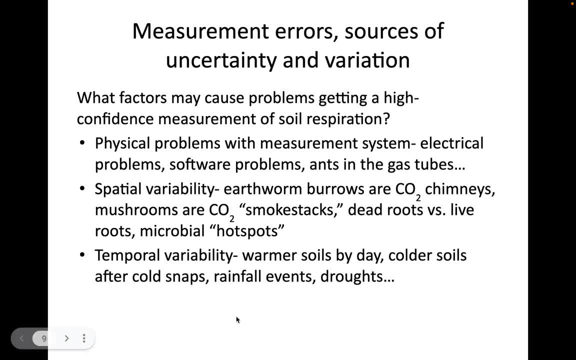 of water, uh, earthworm hot spot um. and then temporal variability as well. um could change day by day, right? um, as organisms you know take advantage of warmer temperatures um and then also throughout the year. right, you might have differences in climate and we'll actually see how that changes. 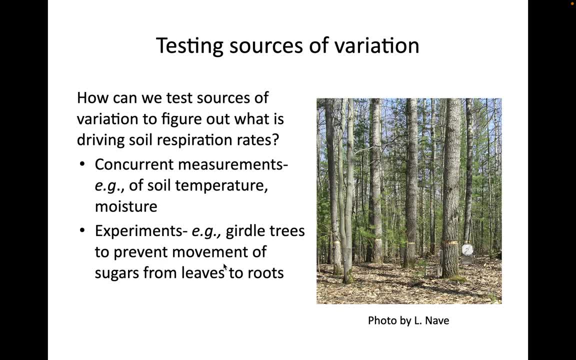 through the year, um. so here's a couple examples of like some experiments you could do, basically so taking multiple measurements. so we're measuring the respiration, but we're also measuring the soil temperature, we're also measuring the moisture, seeing if there's a correlation between any of those, or doing a type of experiment. so in this case they girdled. 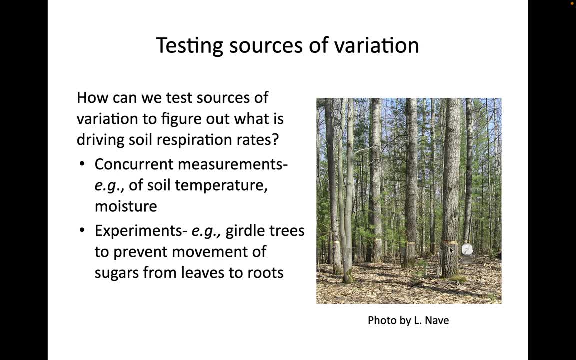 the trees, and so this doesn't allow nutrients to pass up through the tree, but allows the tree to keep standing um, and that's a really important point, right you? you could cut down the trees and that would have the same effect, but then maybe the trees wouldn't have the effect of holding. 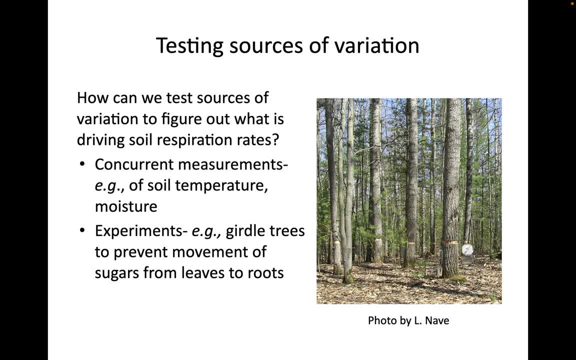 the soil in, and then you would kind of compound your issue. so right now all we're doing is we're stopping the flow of nutrients. we're not stopping the roots, holding the soil in place and that type of thing. girdling is really cool. we actually did a girdling project at prescott college. 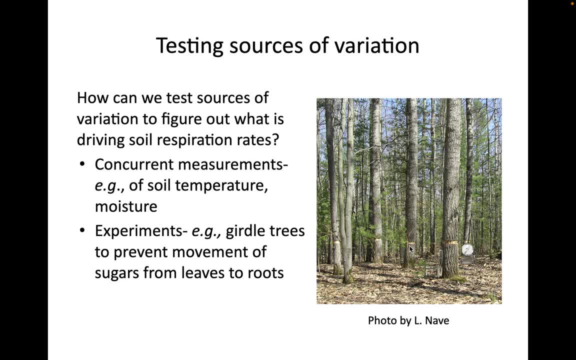 there's some invasive elms that live along that's butte creek and we wanted to replace the ums with some nice willow and cottonwood- and you know there's nice birds that live in the trees, so you don't want to just cut them all down. 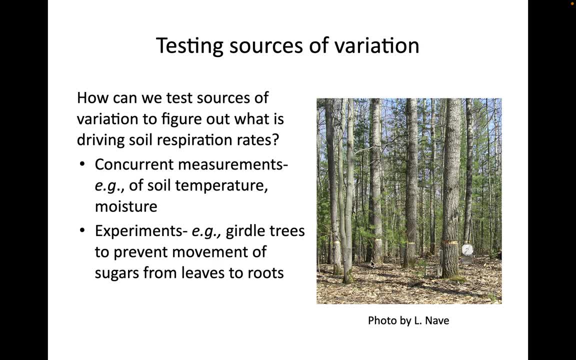 so we ended up girdling some and that way, when the tree is dead, it still is a good habitat, still provides great food source, and then that also allows the little baby trees to grow up. at the same time there's a. this little trail is is going to do great now that these 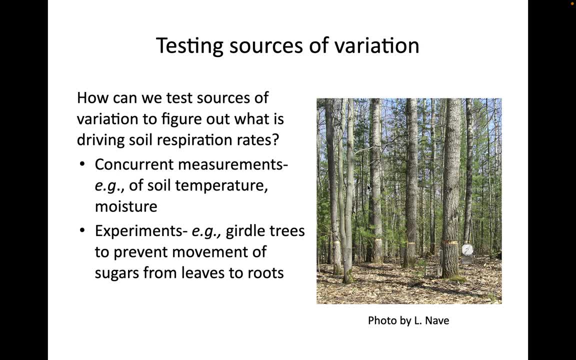 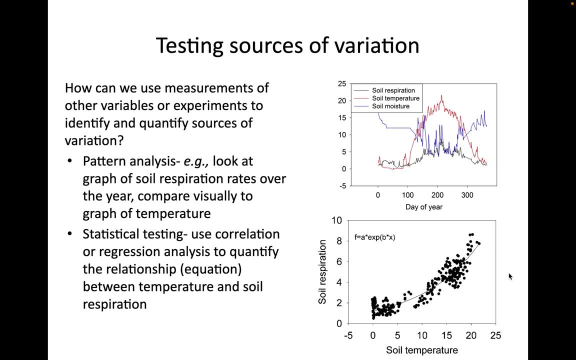 bigger ones will be moving out of the way. a little bit of secondary succession happening right there, um, and so this is, uh sort of an example of the two graphs that you are going to strive to make here. so, looking at soil respiration compared to temperature and moisture.